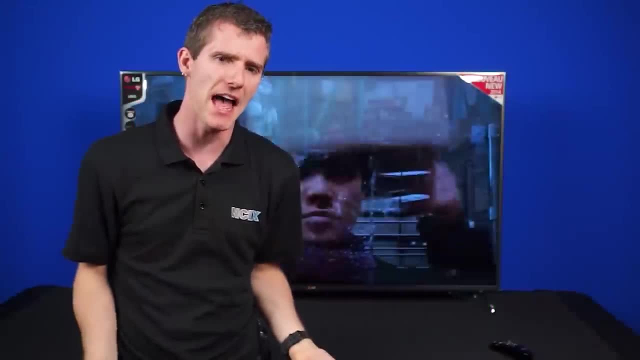 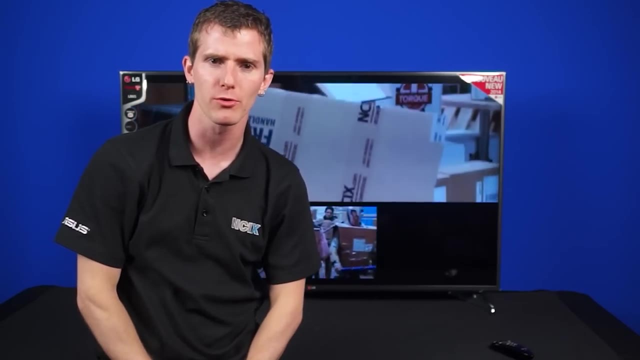 to you. Traditionally, smart TVs were very bad at multitasking. Using any apps or features meant that an ugly full-screen UI would completely cover up the show you were trying to watch. As a result, many people tended not to use these apps at all. 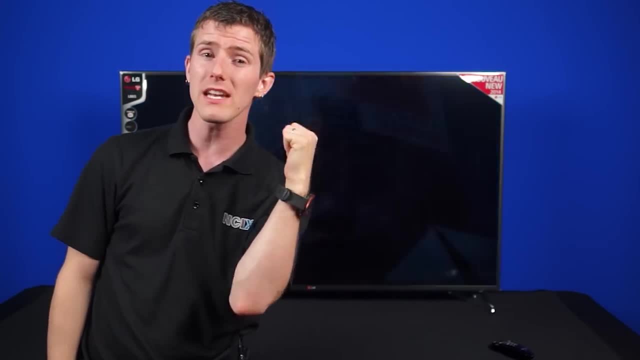 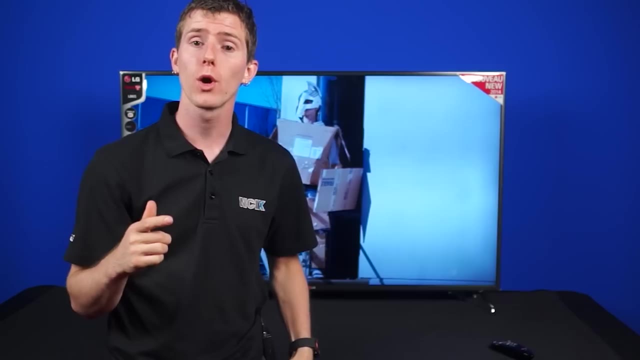 The new webOS interface is designed to use as little of the screen as possible, while still giving you all of the vital information and leaving your show on in the background. Furthermore, with the beefy multi-core processors and higher memory amounts on the latest models, you can now multitask. 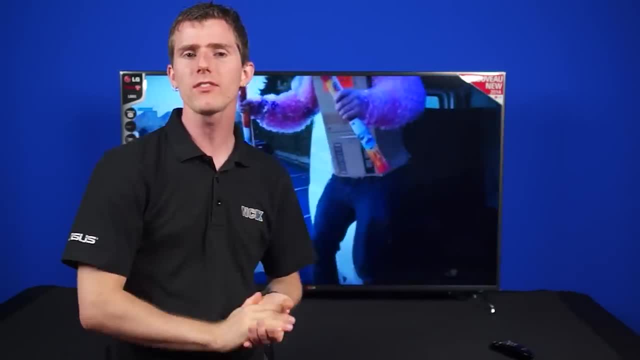 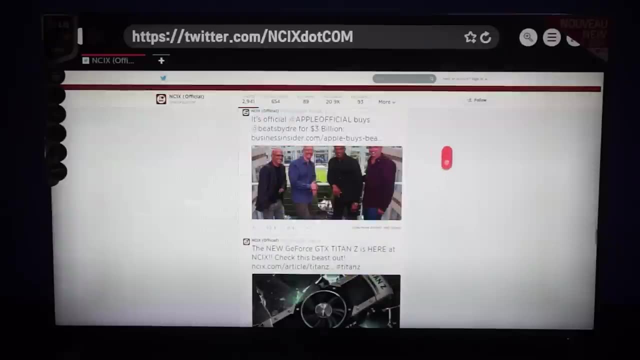 Yay. Multitasking with a TV WebOS allows you to run multiple apps without closing them right away, similar to Android phones. So, for example, you could switch to Twitter during a commercial break, read a funny tweet, share it with your friends on Facebook and return to the show right at the end of the ads. 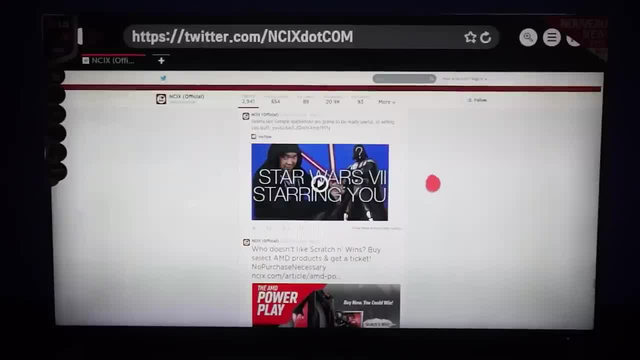 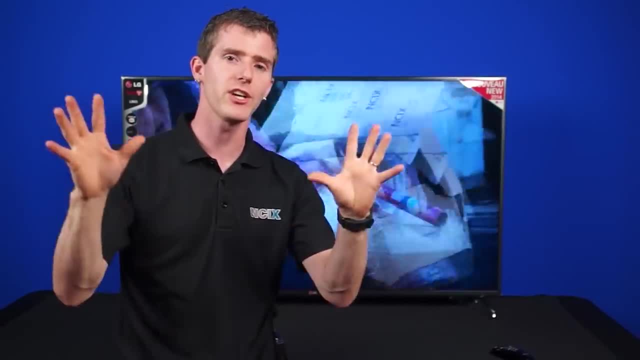 Or you could get a snack. I mean, there's lots of things you can do during commercials other than watching them. It's like Yay. Lastly, webOS has complete integration with LG's magic remote, which features four different methods of input. 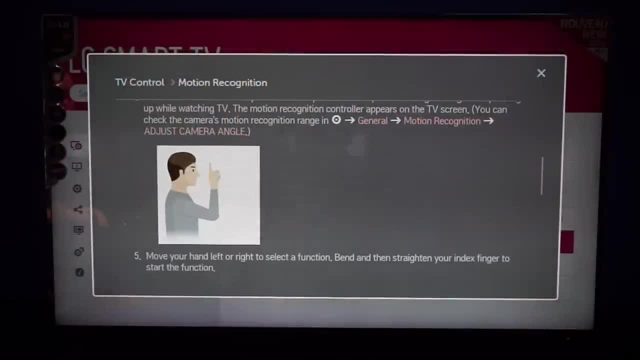 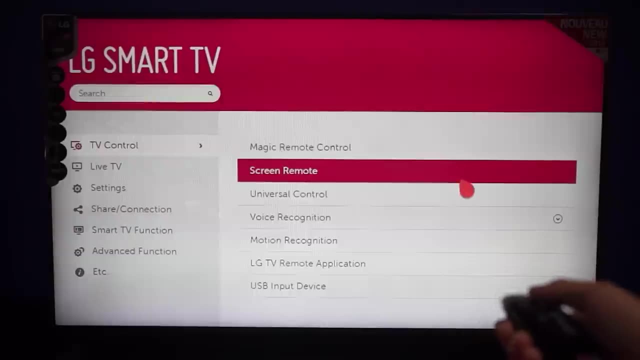 Armed with gesture control, you can program easy gestures, such as swipes, shakes or directions to perform common tasks such as switching channels or volume control. Next, you can simply aim and click at objects on screen, similar to a Nintendo Wiimote. 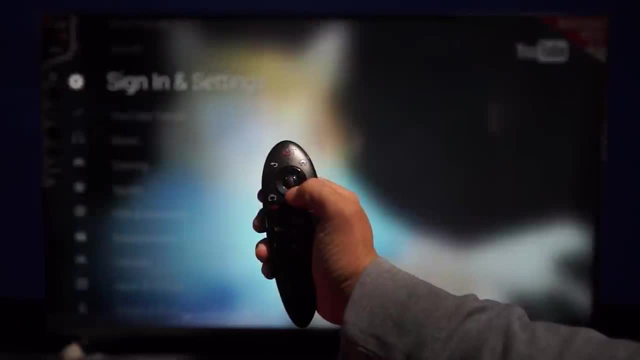 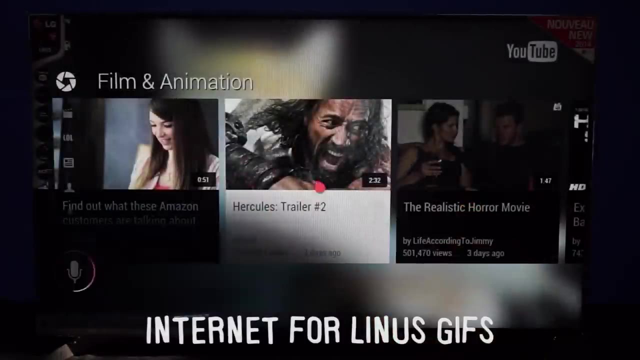 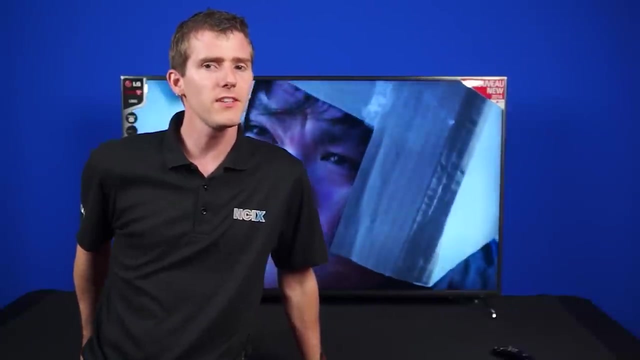 If you prefer the traditional style of control, there's still a four-way D-pad Or, last but not least, you can even use Siri-style voice command type of interface so you can ask it simple questions or give it commands. Overall, on our LG 55-inch LB6500,, we found the user experience very positive. 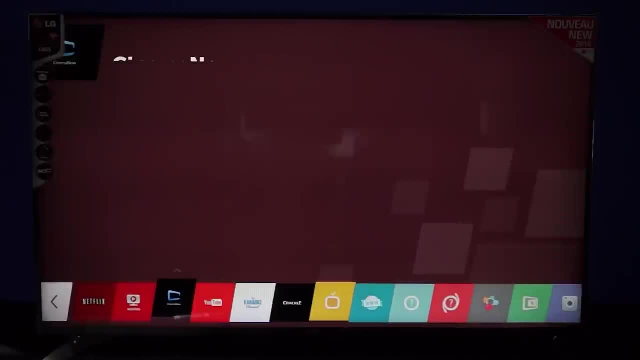 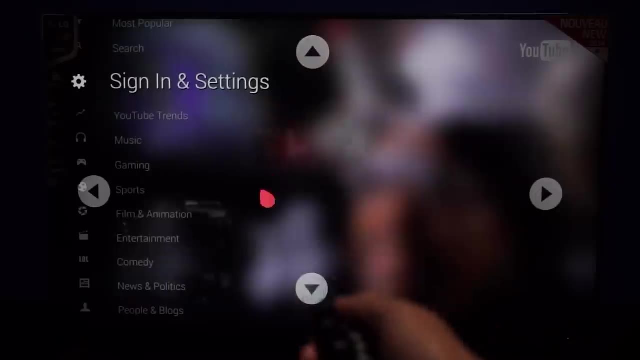 Menus popped up quickly, their animations were smooth and, most importantly, our viewing experience was not completely interrupted by trying to use the smart features. The magic remote controls were quite responsive and the aim and point mode tracked the remote perfectly. The voice commands were probably the least convenient. 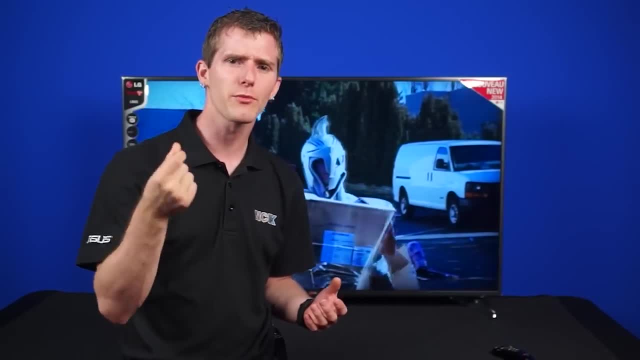 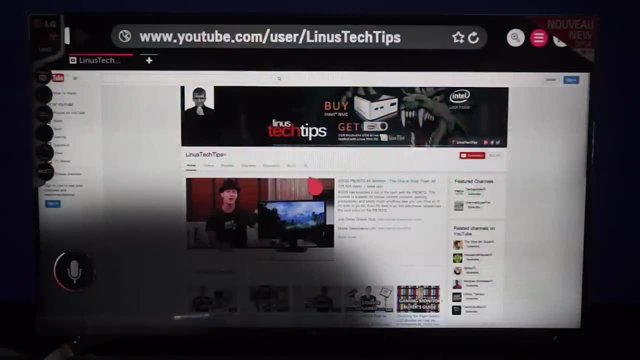 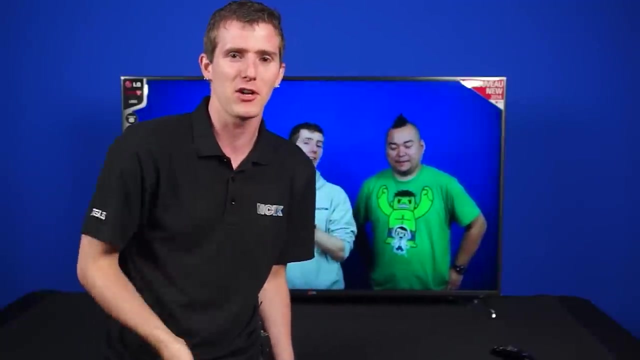 Um, As I would want pretty nearly an instant response when controlling a television. So, for example, if you tell it to adjust the volume, you might have a few steamboats that you can count in between it actually happening. So I mean, sometimes, depending on the kind of show that comes on, you might need to adjust that volume pretty quickly.